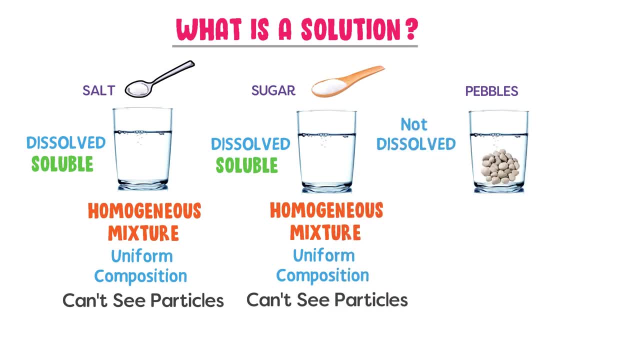 the water, a non-uniform composition By homogeneous mixture. I mean that we cannot spot or see the particles of sugar and salt with naked eye. Solidugar I, minute 1, palabra 甜 21 of pebbles and water with necked eye. Now listen carefully. Salt and water are soluble in each. 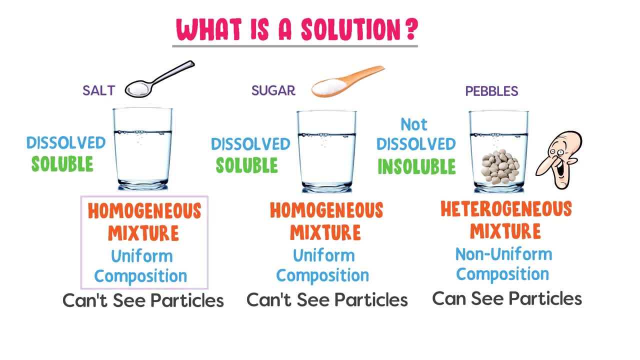 other to form a homogeneous mixture, So it is a solution. Secondly, sugar and water are also soluble in each other to form a homogeneous mixture, So it is also a solution. Thirdly, pebbles are insoluble in water and they form a heterogeneous mixture, So it is not a solution. 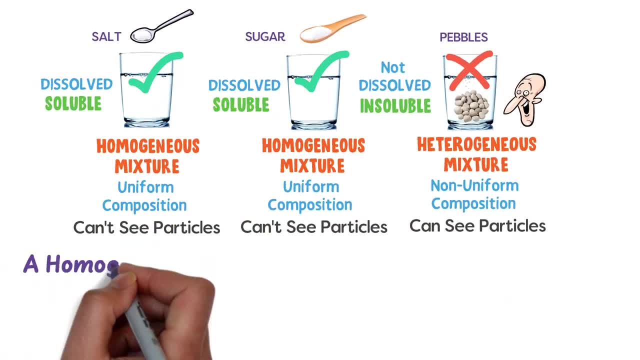 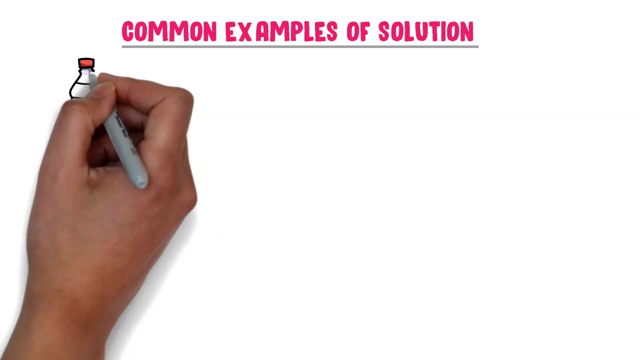 Therefore, we define a solution as a homogeneous mixture of two or more substances is called a solution. Let me repeat it: A homogeneous mixture of two or more substances is called a solution. Now let me give you some common examples of a solution. Well, the first example of a solution is cold drinks. In cold drinks, 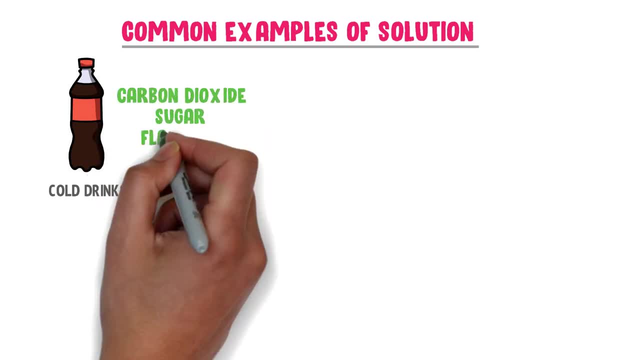 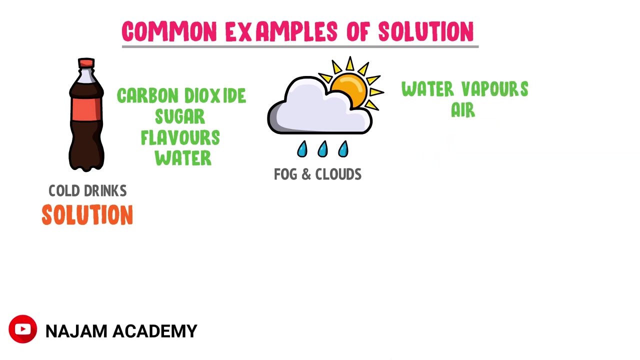 carbon dioxide, gas, sugar and flavors are dissolved in water to form a homogeneous mixture or a solution. Secondly, fog or clouds, Water vapors dissolve in the air to form a homogeneous mixture or solution. Thirdly, smoke and the air: Carbon particles dissolve in air to form a homogeneous mixture or a solution. 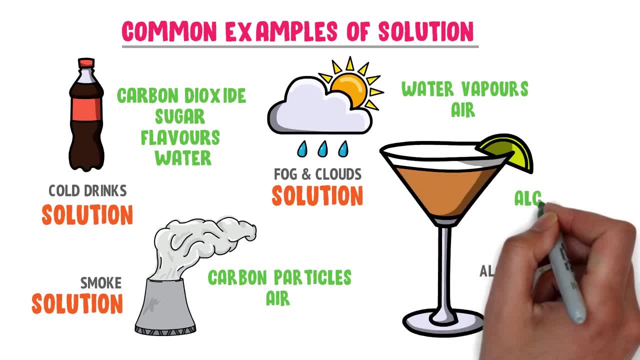 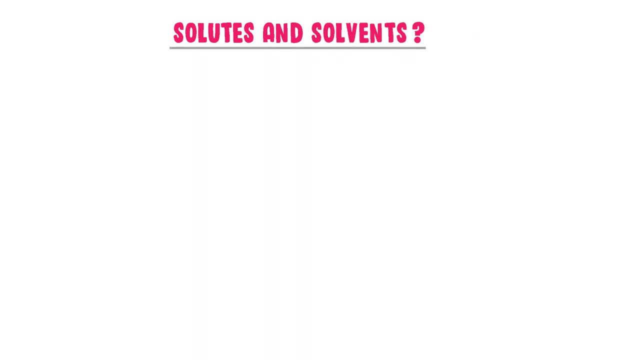 Fourthly, alcohol plus water. Alcohol is dissolved in water to form a homogeneous mixture or a solution. So these are the common examples of a solution. Now, what are solutes and solvents? Well, let's consider a salt solution, a sugar solution. we know that in a salt solution there are two components: salt. 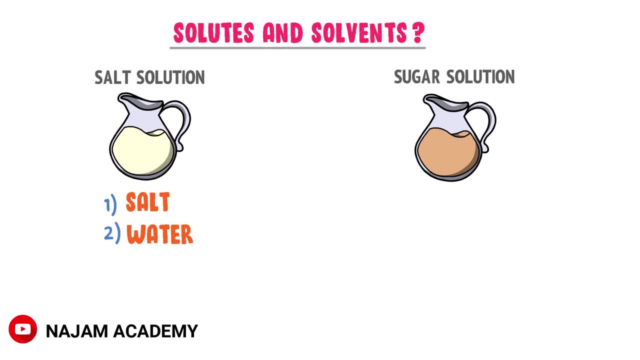 and water, while in sugar solution there are also two components: sugar and water. secondly, we also know that in salt solution, salt is dissolved in the water, while in sugar solution, sugar is dissolved and water. thirdly, in salt solution, salt is present in smaller quantity and water is present in larger. 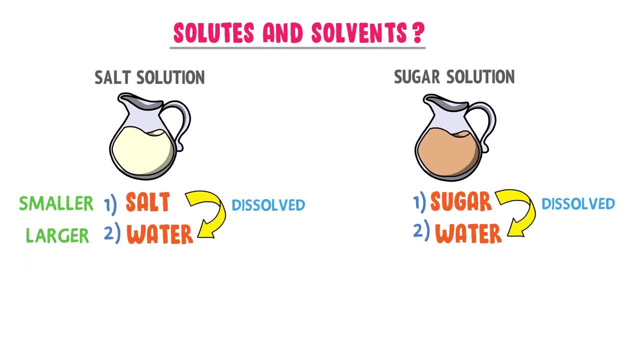 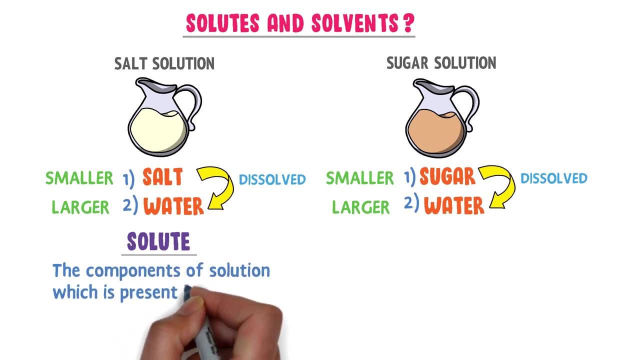 quantity, while in sugar solution, sugar is present in smaller quantity and water is again present in larger quantity. therefore, we define solute as the component of released solution, and this'll be called like that of a solution which is present in smaller amount is called solute. Let me repeat it. 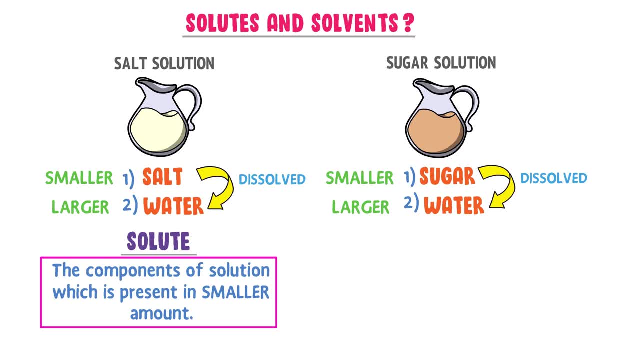 The component of a solution which is present in smaller amount is called solute, While we define solvent as the component of a solution which is present in larger amount is called solvent. Let me repeat it: The component of a solution which is present in larger amount is called. 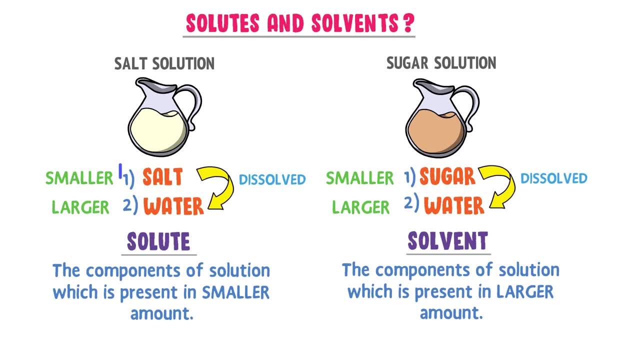 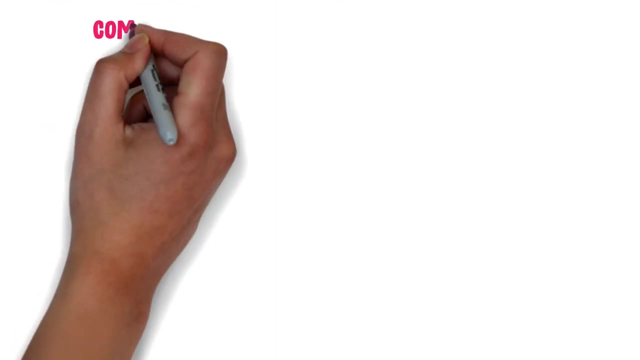 solvent. So in salt solution, salt is a solute because it is present in smaller amount, and water is a solvent because it is present in larger amount. In sugar solution, sugar is a solute because it is present in larger amount. Now let me give you some common examples of solute and solvent. Well, consider a solution of 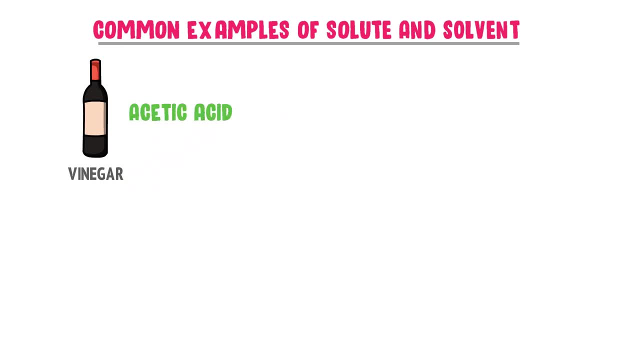 vinegar. In vinegar, acetic acid is dissolved in water, So acetic acid is a solute and water is a solvent. Secondly, a solution of vinegar is called solvent because it is present in larger amount. Now let me give you some common examples of solute and solvent. Well, consider a solution of sugar and milk.